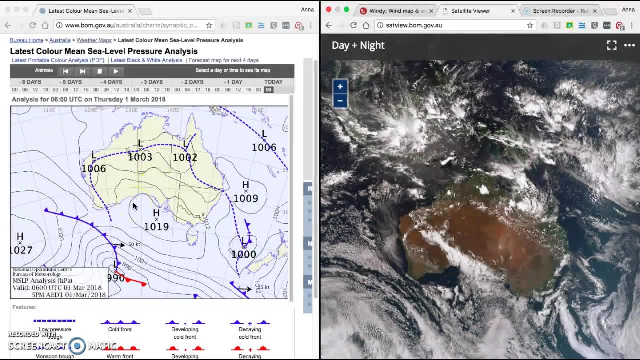 the first thing you need to know, And you would know from previous lessons, that the closer the isobars are, the stronger the winds. So the closer the isobars, the stronger the winds, And the winds in general like to move anti-clockwise around the high and clockwise around the low. 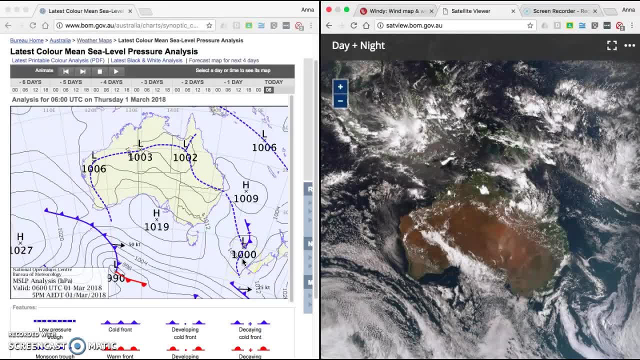 in the southern hemisphere It's different in the northern hemisphere. Okay. so these H's, they stand for a high pressure system, So it's the places of highest pressure in the local area. Okay, and winds in the high pressure move away, they descend, It's cool. 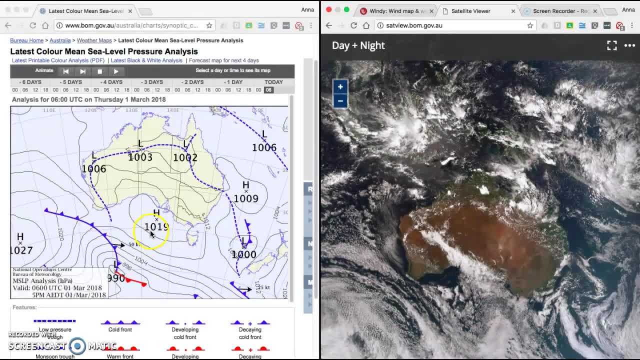 dry winds. So it's dry weather. This is what we expect from here- And they're descending and they're moving away, Okay, and in general, they move towards the low pressure system. So here in New Zealand we have a low, We also have some lows. 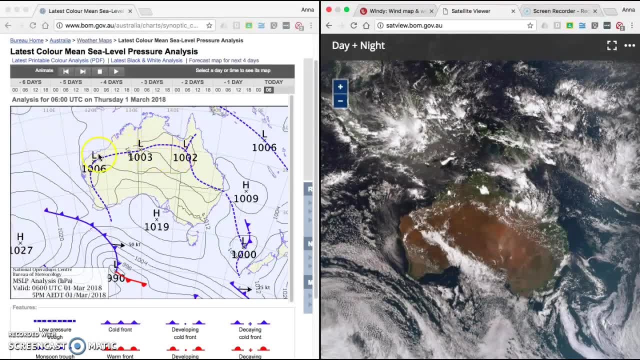 in the northern part of Australia, but I want to particularly point out this one. Okay, so this is the lowest low in the northern part, Alright, so these lows you should remember from previous classes. this is where the wind is moist and warm and it rises. 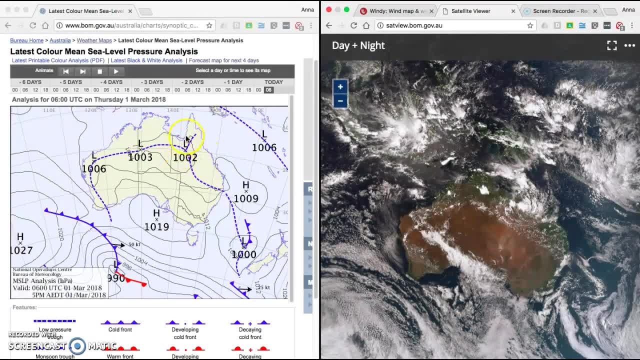 It expands and it rises And when you have moist warm air expanding and rising, you usually get clouds, You get cloud coverage. So that's what's happening in a low And remember it's moving in a clockwise direction. the winds. 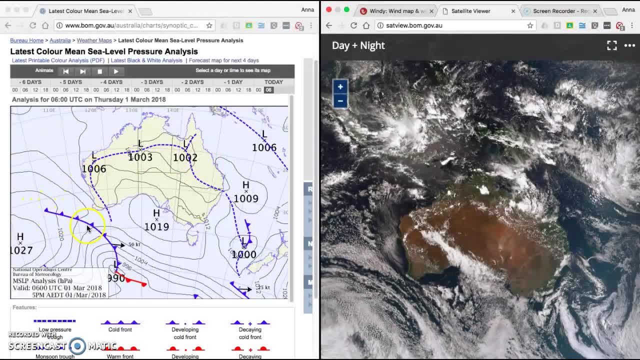 Okay, If we look here, this special line here. you might not have seen that before, But that's called a cold front. This blue line is a cold front And a cold front. not all synoptic charts have colors, but a cold front is symbolized. 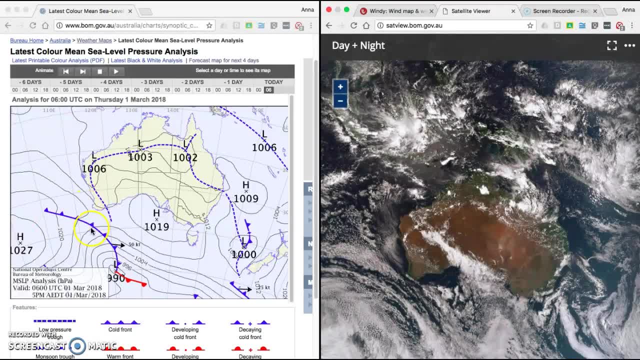 by a line with pointy, with triangles- okay, with triangles. And a cold front is cold, okay, It's cold dense air, And what it does is cold dense air replaces warm air, which is on this side. It's moving in this direction, which is pointed to by the arrow. 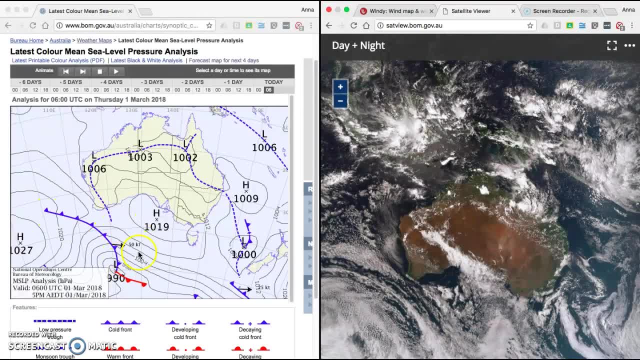 Okay, So a cold air mass replaces warm air. This is what we call a warm front. So this is the opposite. So we have warm air moving and it's replacing cold air. Okay So, warm air replacing cold air. It's the red line and you've got the bumps, not the spikes, the bumps for a warm front. 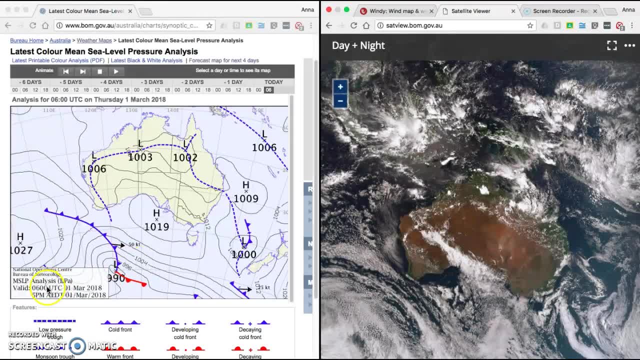 Okay, So these cold fronts in the southern hemisphere come from the south pole, They usually come from the south And they generally, They usually move from a west to east direction. Okay, And the final thing to point out is this broken blue line, this broken blue line. 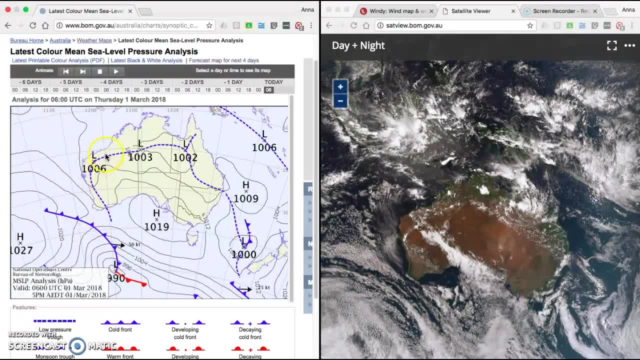 It's nice, It's all across Australia. Okay, So this broken blue line is called a low pressure trough. It's not a low pressure system, It's low pressure trough, And the low pressure trough means there's an atmospheric disturbance And usually with this there's some light cloud cover. 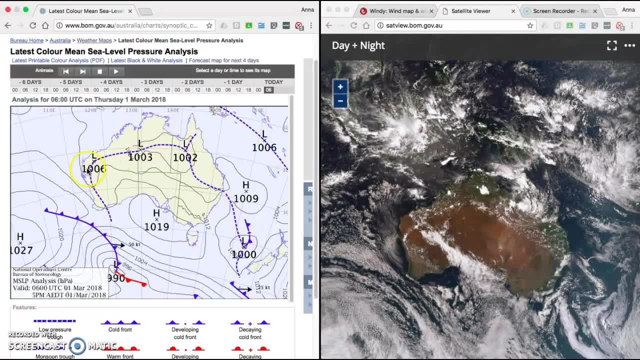 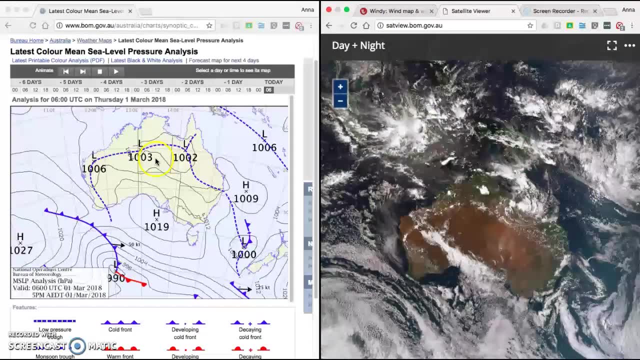 Even rain, And so rain can be associated with this low pressure trough. Okay, So let's look at our map on this side, Okay, And let's look at our synoptic chart, And what you can see is that here in the low pressure system, we're getting clouds. 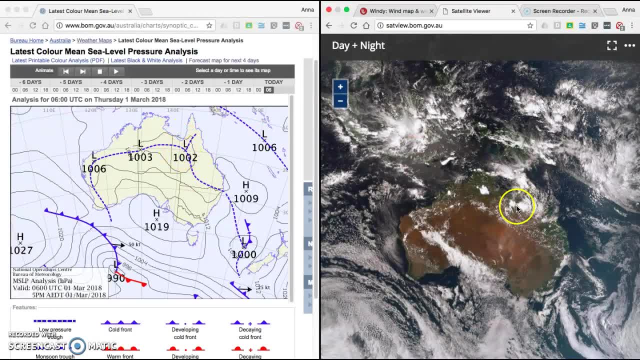 Okay, So it corresponds nicely: Low pressure system, clouds. Now The What we have here Is we have a cold pressure system, We have a low pressure trough going across Australia And you can see that this low pressure trough follows this strange curvy pattern. 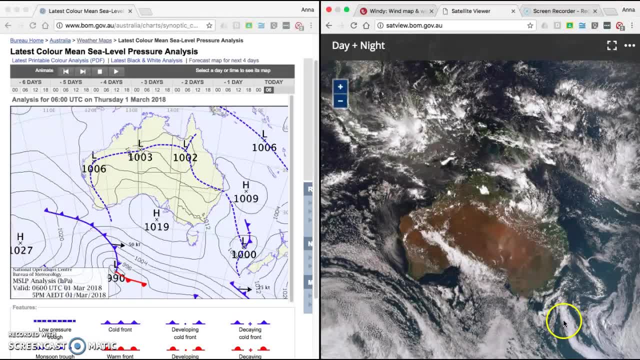 And the cloud cover of Australia follows a similar low curvy pattern. Okay, And in the high areas, where there's none of these low pressure troughs, we have clear areas. Now, yesterday or today. you'll be watching this today. You'll be watching this the day after. 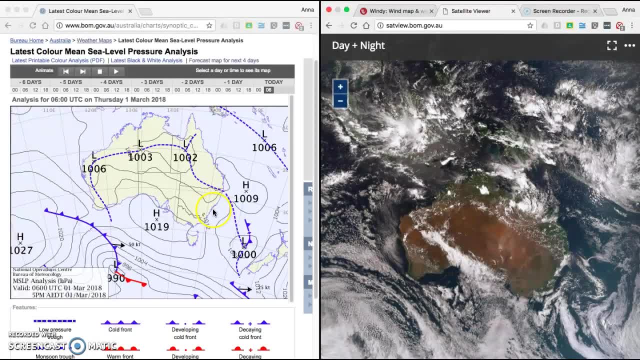 Today in Sydney there was this line. It was actually here earlier at 11 o'clock, And that's when we got cloud cover, So you would have been able to see it if you're watching this on the 1st of March.